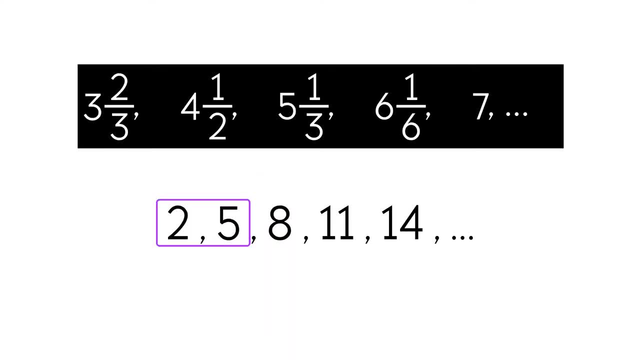 2 and 5.. To find the rule, we can subtract 2 from 5 to get 3.. So the rule is to add 3 for each term. Now let's take a look at another sequence. Unlike the previous sequence, this sequence- 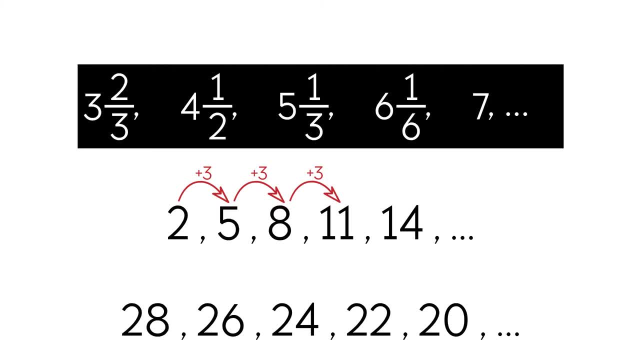 is decreasing, The numbers get smaller. To find the rule, we take a look at two consecutive numbers. we subtract the smaller number from the larger number and we see that the rule is to subtract 2.. Now let's take a look at the sequence of mixed numbers. 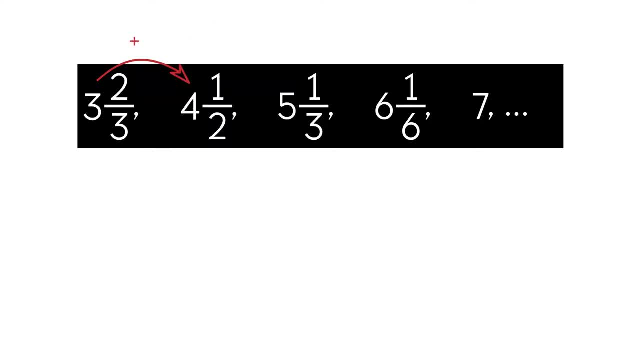 We see that the sequence is increasing because the numbers get larger. Now let's try to find the rule. We take two consecutive numbers, 4 and 1 half, and 3 and 2 thirds. Let's try to subtract them. As you can see, we can't subtract because the denominators 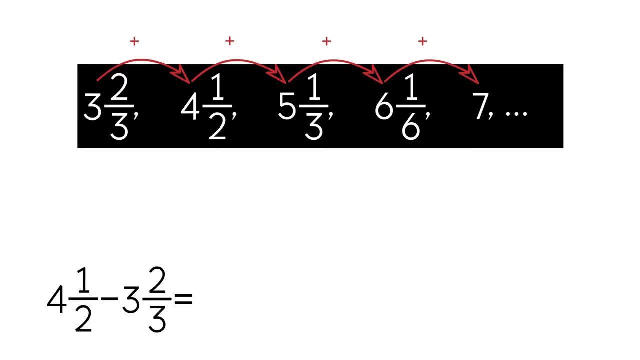 are not the same. We need to find the least common denominator. The least common multiple between 3, 2, and 6 is 6.. So the common denominator is going to be 6.. For the first mixed number, we multiply the denominator and the numerator by 2.. 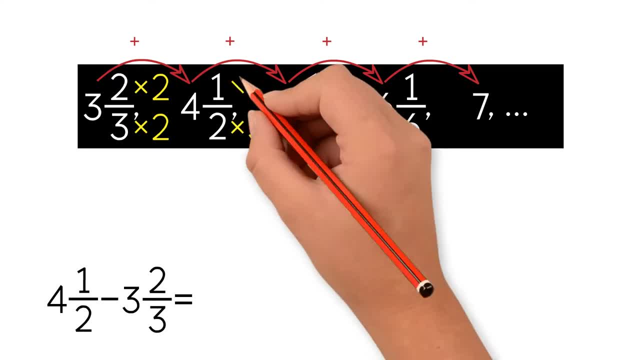 For the second mixed number, we multiply the denominator and the numerator by 3.. For 5 and 1 third, we multiply the denominator and the numerator by 2.. We leave 6 and 1 sixth the same, because the denominator is already 6.. 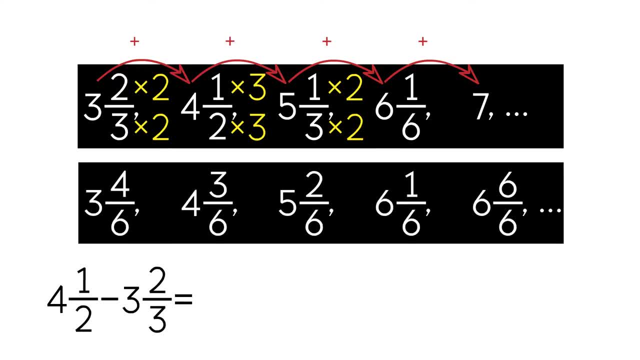 Now we can rewrite the mixed numbers with the equivalent fractions. Now, instead of subtracting 3 and 2 thirds from 4 and 1 half, we subtract 3 and 4 sixths from 4 and 3 sixths. But we run into a small problem. We can't subtract 4 sixths from 3 sixths, So we have 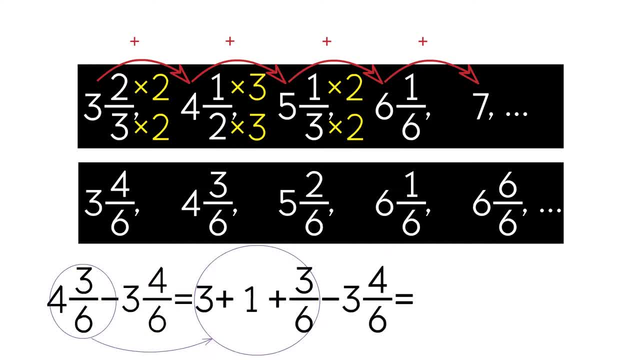 to regroup: Instead of 4, we can write 3 plus 1.. And instead of 1, we can write 6 over 6.. So now our mixed number 4 and 3 over 6 turned into 2.. 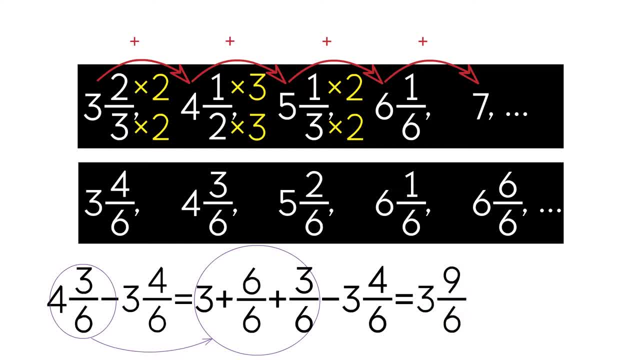 Now let's try to find the rule turned into 3 and 9 over 6.. Now we can subtract 3 and 9 over 6 minus 3 and 4 over 6 equals 5 over 6.. So the rule is to add 5 over 6.. 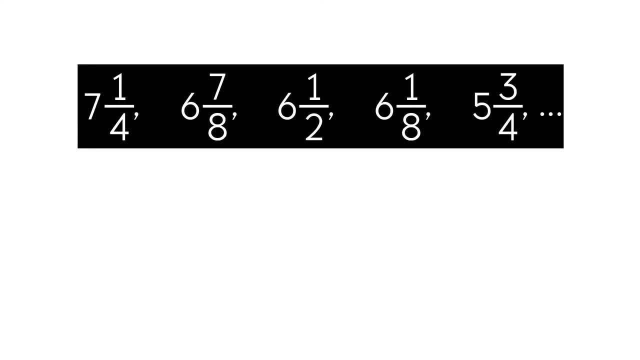 Let's do another example. As you can see, this sequence is decreasing. The numbers get smaller. To find the rule, we need to take two consecutive terms. We subtract the smaller term from the larger term and we get the rule. Let's take 7 and 1. fourth, 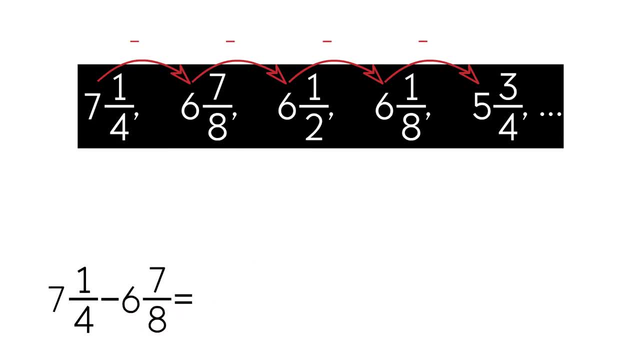 minus 6 and 7 eighths To subtract, we're going to need a common denominator. We have the denominators 4,, 8 and 2.. The least common denominator between those numbers is 8.. We multiply the denominator and the numerator of the first fraction by 2.. 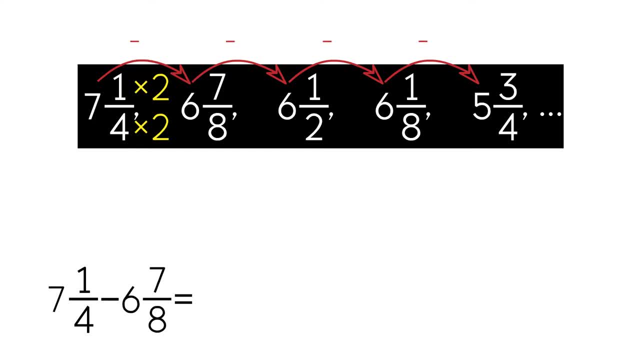 We leave the second term the same, because the denominator is already 8.. For the third term, we multiply the denominator and the numerator by 4.. We leave 6 and 1 eighth the same, because the denominator is already 8.. For the fifth term, we multiply the denominator and the numerator by 2.. 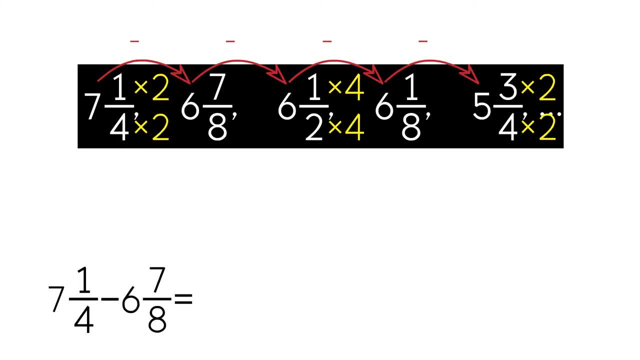 We actually didn't need to rewrite every single mixed number to have the denominator of 8. We did that just for educational purposes. We really only needed to do that for two consecutive terms that we're going to subtract. So now we have a new sequence. 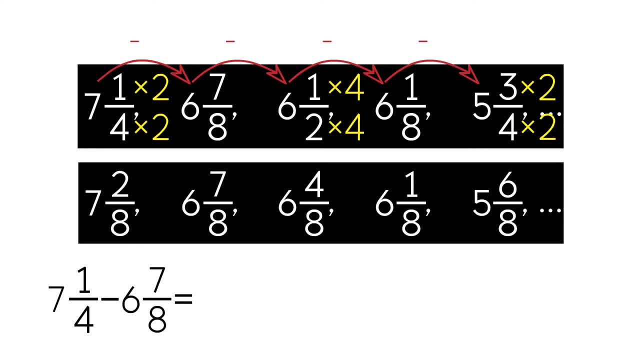 where all of the denominators are 8.. Now we can rewrite the original equation to 7 and 2 eighths minus 6 and 7 eighths. We can't subtract 7 eighths from 2 eighths. 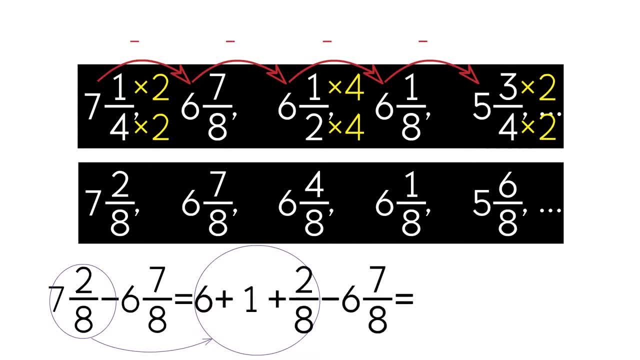 so we have to regroup. We rewrite 7 as 7 and 2 eighths. We can re-write 1 as 6 plus 1.. And we rewrite 1 as 8 over 8.. We can rewrite 7 and 2 eighths to 6 and 10 eighths. Now we can subtract. 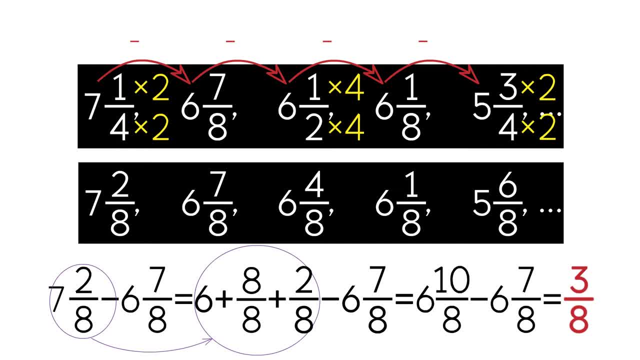 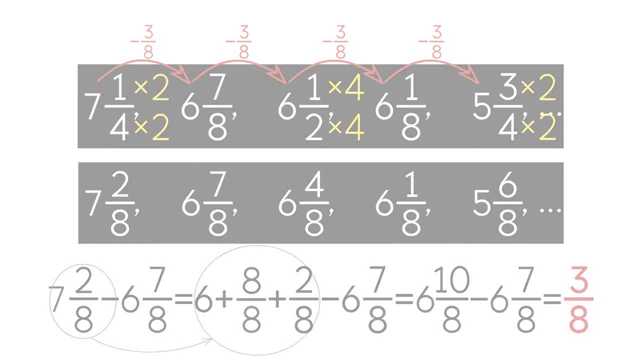 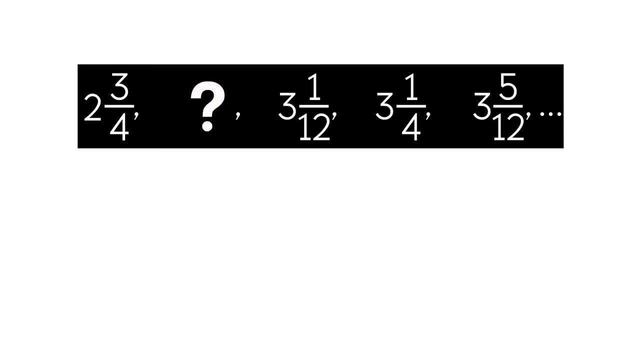 We subtract and we get 3 eighths. So the rule is to subtract 3 eighths. Let's do a different example. We have an unknown term. To find the unknown term, we need to find the rule for the sequence. We can see that the sequence is increasing.